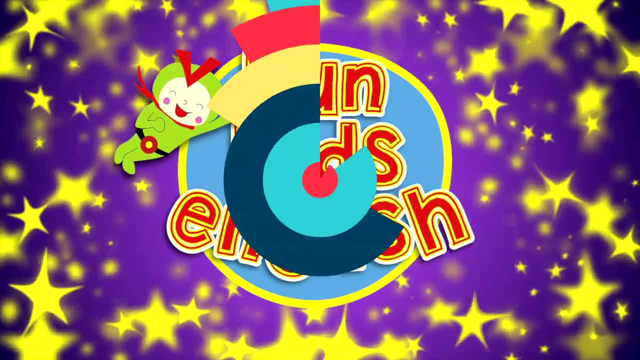 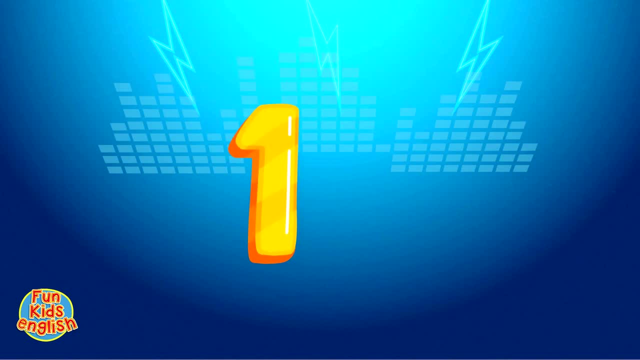 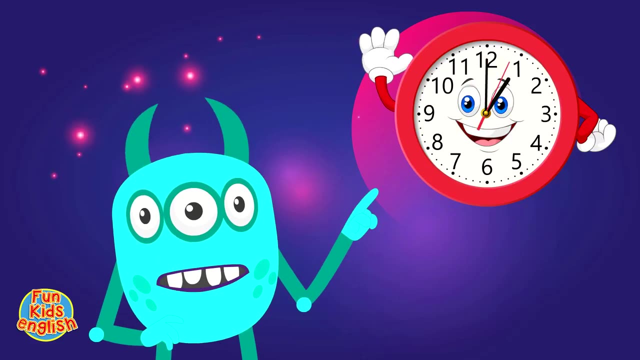 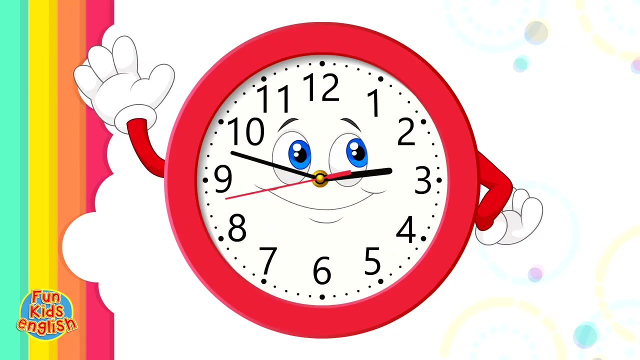 5,, 6,, 7,, 8,, 9,, 10,, 11,, 12,, 13,, 14,, 15,, 16,, 17,, 18,, 19,, 20,, 21,, 22,, 23,, 24,, 25,, 26,, 27,, 28,, 29,, 30,, 31,, 33,, 34,, 35,, 36,, 37,, 38,, 40,, 40. 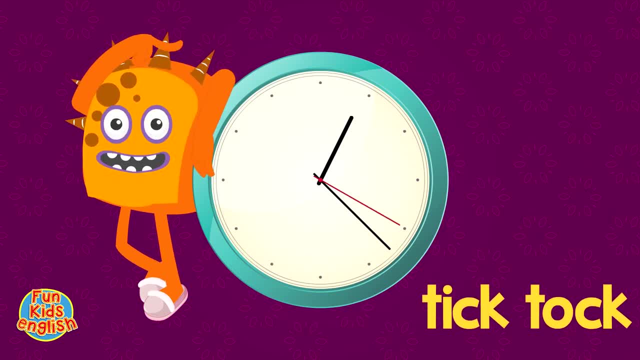 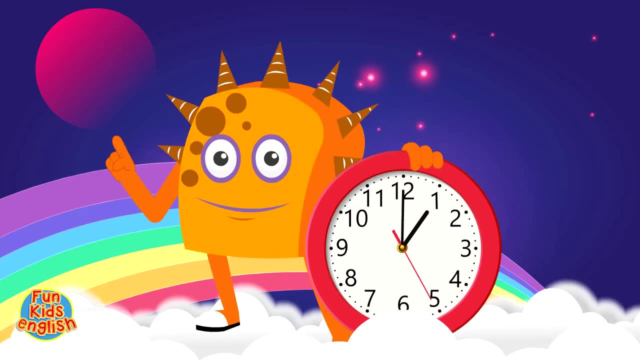 The clock says tickety-tock, tick-tock, tick-tock, tick-tock. Can you help me tell the time? Let's all count from 1 to 12.. Can you help me tell the time? Help me tell the time. 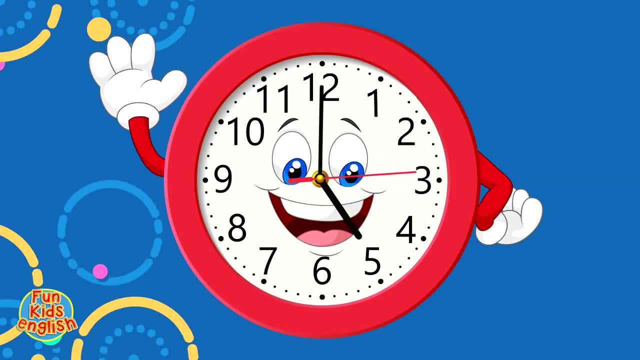 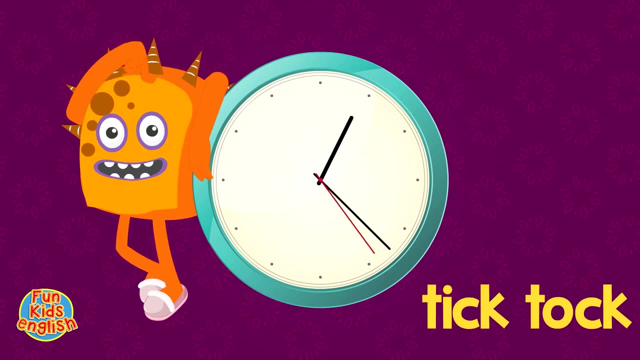 What time is it? It's 5 o'clock, 6 o'clock, 7 o'clock. What time is it? It's 8 o'clock. The clock says tickety-tock. tick-tock, tick-tock, tick-tock. 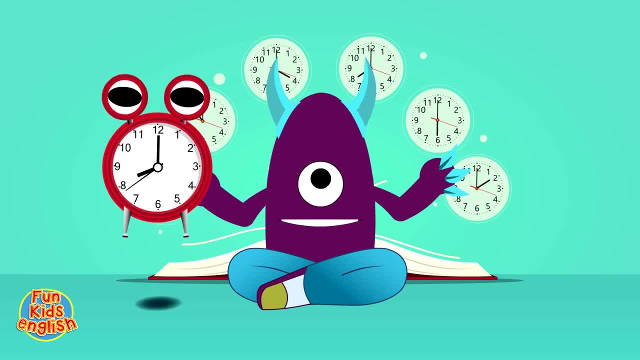 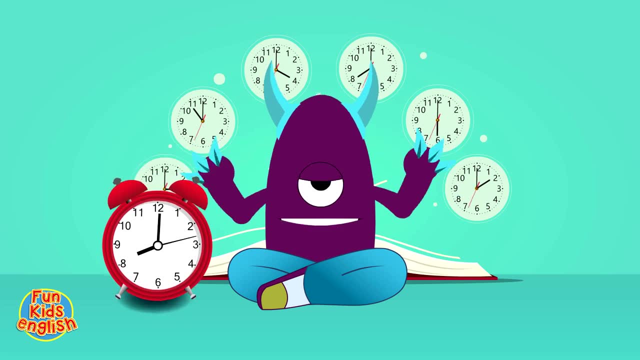 Can you help me tell the time? Let's all count from 1 to 12.. Can you help me tell the time? Let's all count from 1 to 12.. Can you help me tell the time? Help me tell the time. 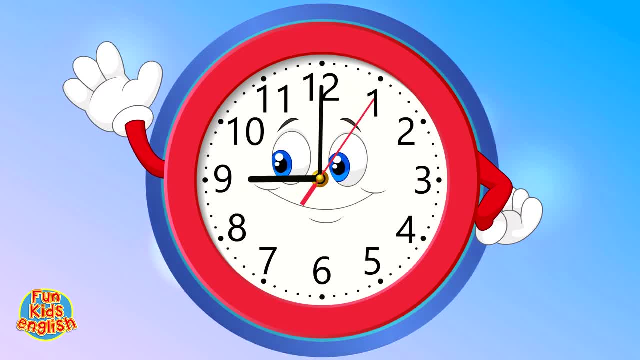 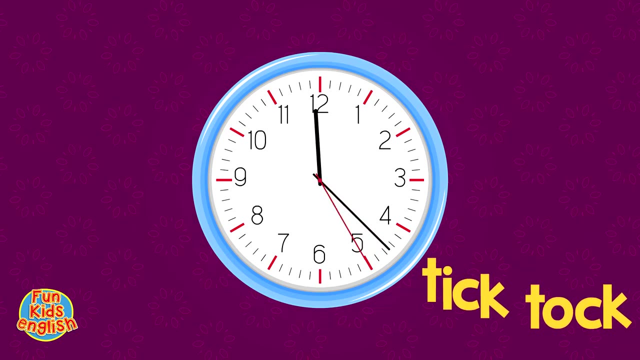 What time is it? It's 9 o'clock, 10 o'clock, 11 o'clock. What time is it? It's 12 o'clock. The clock says tickety-tock. tick-tock, tick-tock, tick-tock. 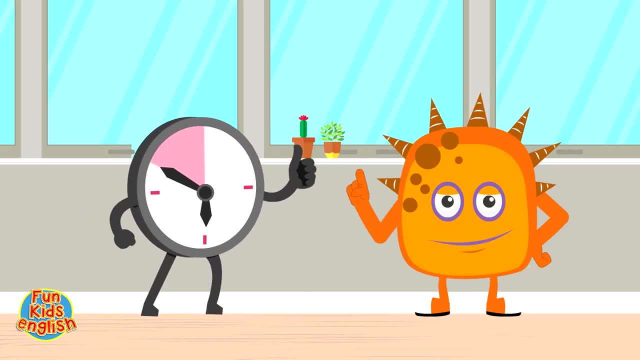 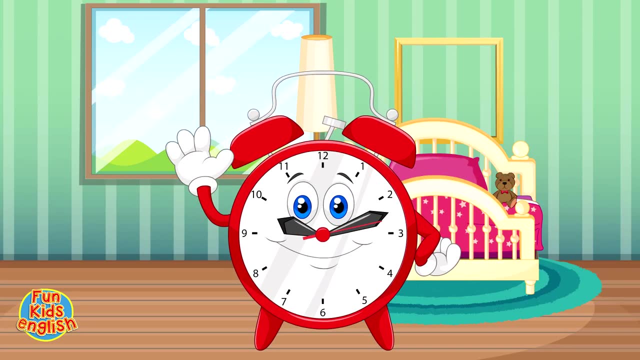 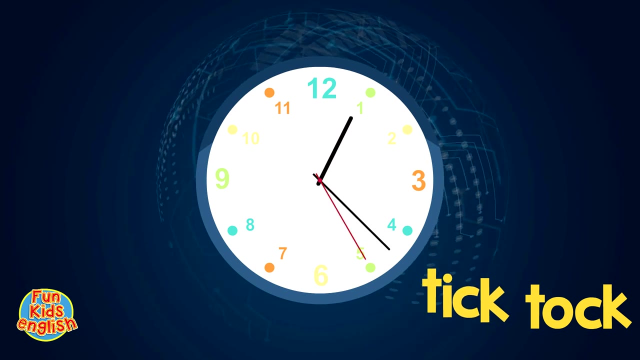 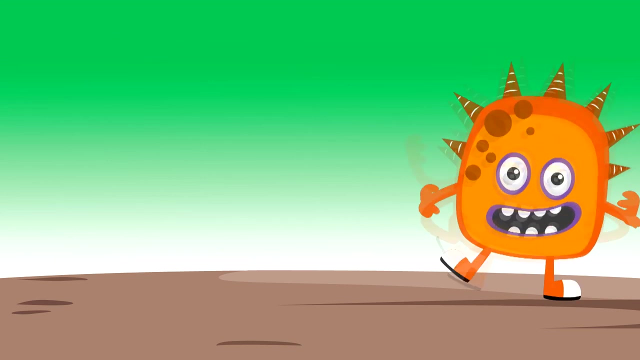 Now we've learnt to tell the time. Everything's fine, We can tell the time. Now we've learnt to tell the time. The clock says tickety-tock, tick-tock, tick-tock, tick-tock. The clock says tickety-tock, tick-tock, tick-tock, tick-tock, tick-tock. 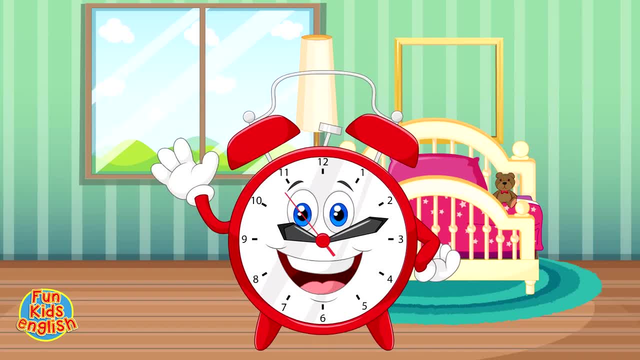 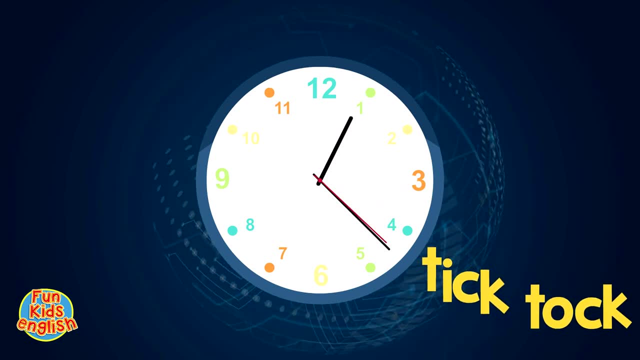 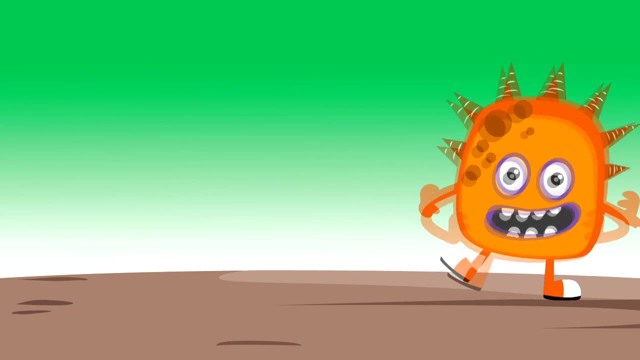 we can tell the time. Now we've learnt to tell the time. The clock says tickety-tock, tick-tock, tick-tock, tick-tock. Now we've learnt to tell the time. 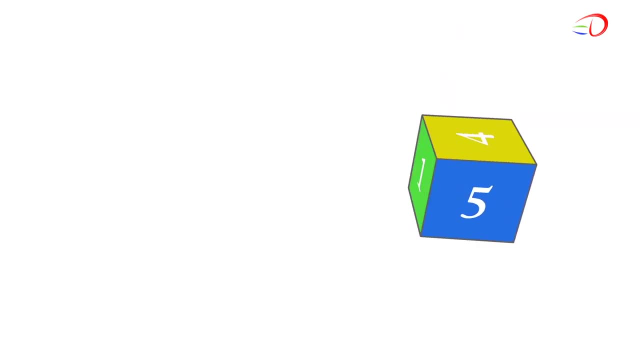 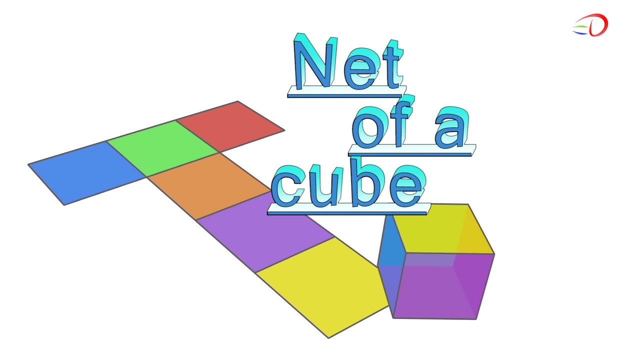 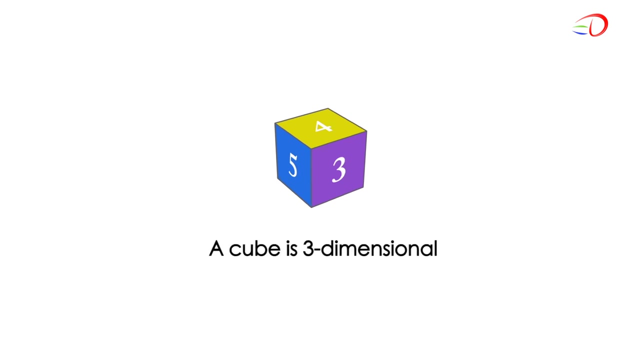 What is the net of a cube? A cube is three-dimensional. If we open up a cube and lay it flat, we'll see that there are six square faces: One, two, three, four, five and six. This is a net of the cube. 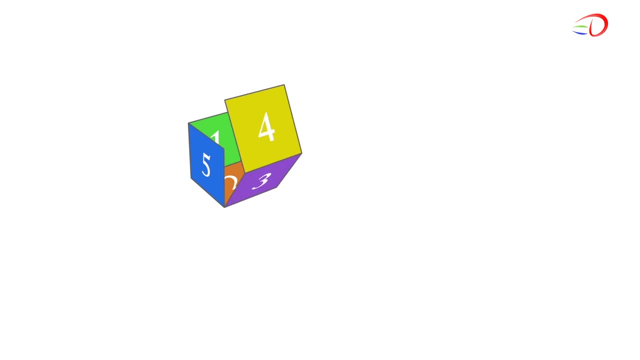 A net is two-dimensional. It can be folded to make a three-dimensional cube. How about this? Can it be folded to form a cube too? Yes, it can. Here is another. Is this a net of a cube? Let's check it out. 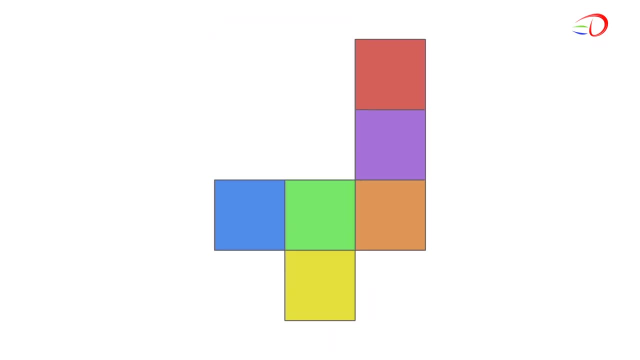 Yes, this is the net of a cube. How about this? Is this a net of a cube too? There is an overlapping face, so this is not a net of a cube. We now know that these are nets of a cube, And we know this is not a net of a cube. 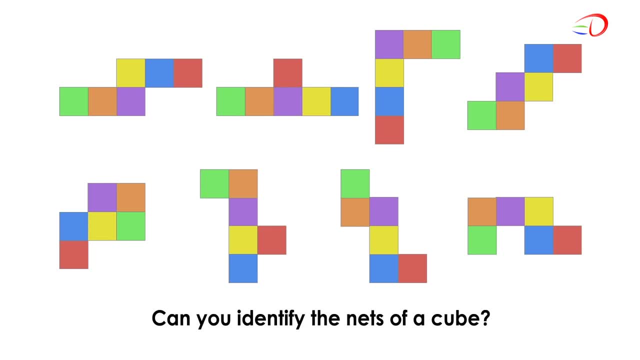 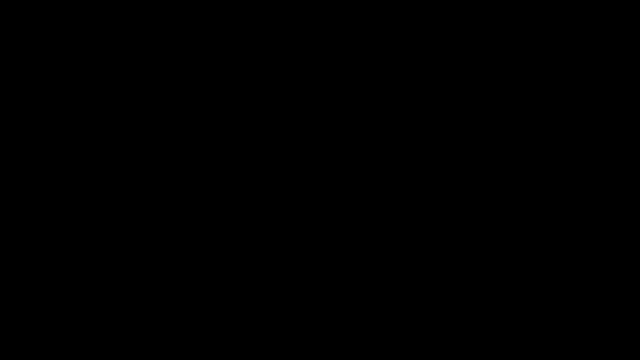 What about these? Can you identify the nets of a cube? Wow, these are the net of a cube. Yes, the net of a cube. Then let's see: How about this? Here's a net of a cube. How many can you find? The net of a cube is one, so this one can be one and the other one is a new. How many can you find Here? I'm going to take some of these Now. let's see. Can you find the inside out?